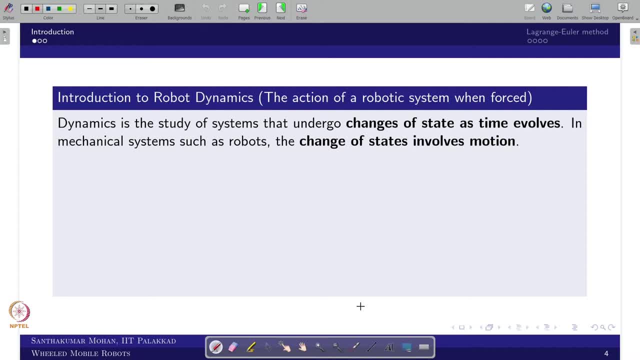 is actually like very broad, where you call actually like it is actually like contradict, or you can say contemporary to the statics, where the statics is actually like nothing but the you call there is a no motion, or the motion with the constant right, or you can. 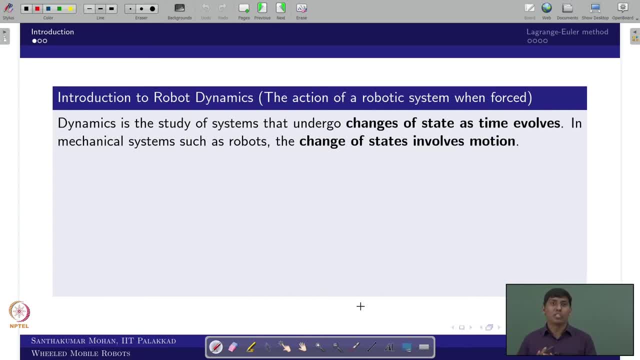 say constant motion, Whereas the dynamics means it is actually like change with respect to time. So here robot dynamics means it is slightly different, because the dynamics is already have a two classification, which we used to do in physics: One is kinematics, the other. 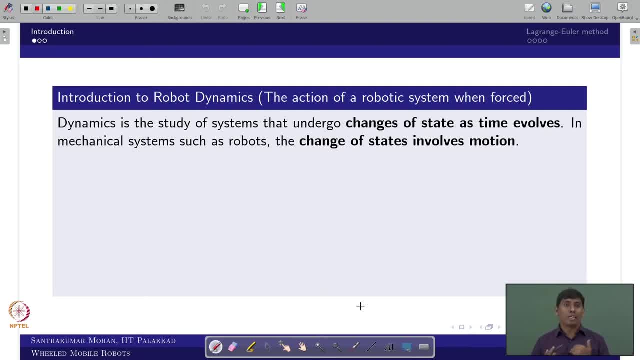 one is kinetics, but here the kinetics we are going to call more general as dynamics. Why it is so? Because dynamics means what the study of motion with respect to what you call change in, you can say inputs, or you can say by incorporating the input In the sense. 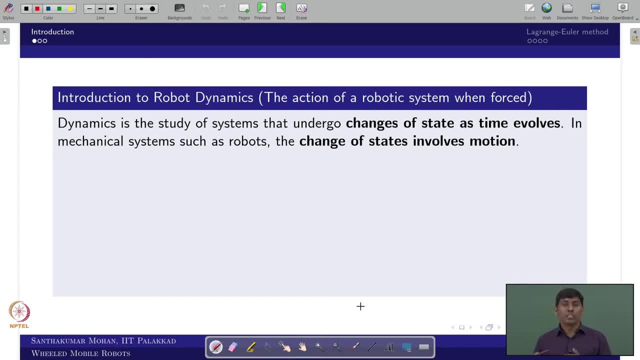 we are seeing the motion with the cause of motion. So then you can see, in robot Dynamics or in mechanical engineering, the kinematics will give the study of motion, but when you talk about dynamics the study of motion is by default incorporate. For example, 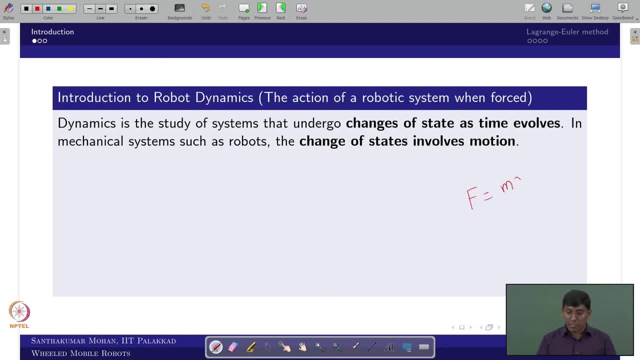 if I write the equation F equal to M, A, so where the A is actually like required, then only I can find the F right. So in the sense, if I give F, I can find A. This is the study of motion. I am relating with the kinematic aspect, For example, if you recall your second, 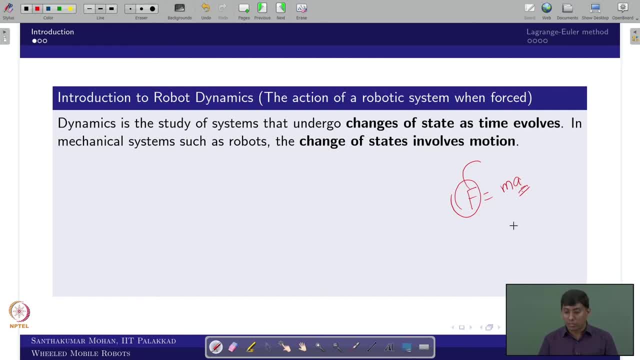 order system response. For example, I have given the second order system response. For example, I am taking a mass spring damper system. just for understanding I am actually taking this is a mass spring damper. So what you use to write the equation: if I give a force F, So this would get displaced. 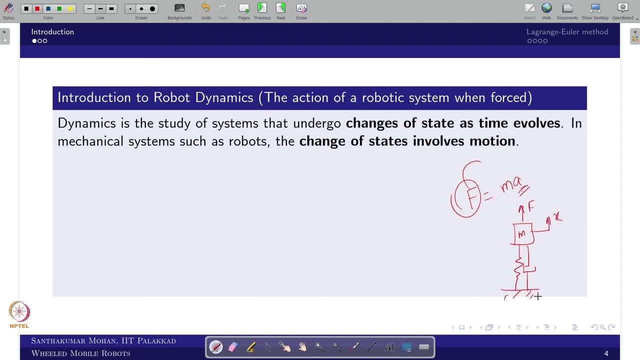 in x. I assume that is one dimensional, where it is only going to move in. you can say upward and downward direction. I call this is the. B is the damping constant and K is, you can say stiffness. So you use to write the F is the input that you would be writing in. 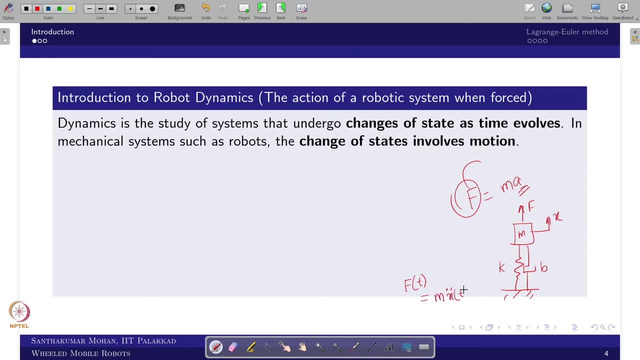 the form of, You can say, You can say time, derivative of the displacement right, So zeroth, and first and second derivative, the sense B, x, dot of t plus K into x of t. So what, in that sense you will try to write. 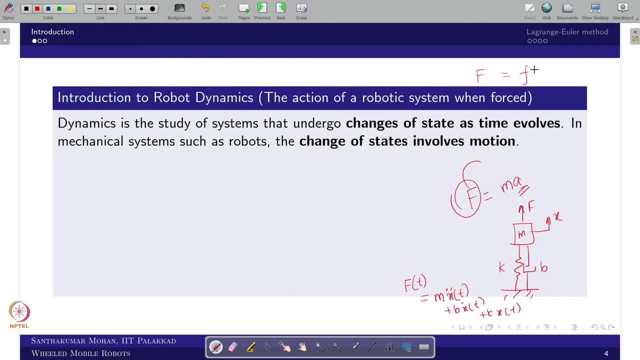 you can say one side, F, So other side is actually like function of x, x dot and x double dot. But what is this? we have studied, We have studied. this is nothing but kinematic aspect. This is what you have seen as a kinematics, But now you are bringing the cause of motion. 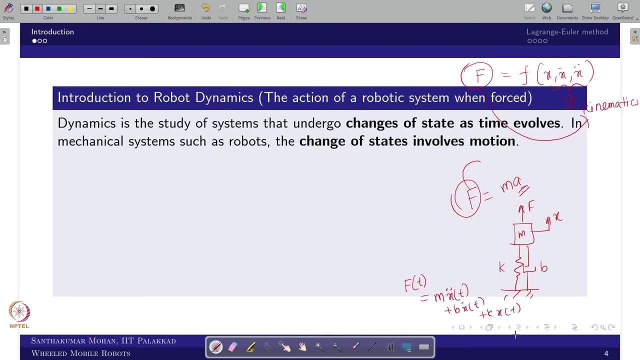 So what we are actually trying to bring? So you are trying to bridge the cause of motion to the study of motion. So that is what you have to see as robot dynamics. So, in the sense, the action of the robotic system. 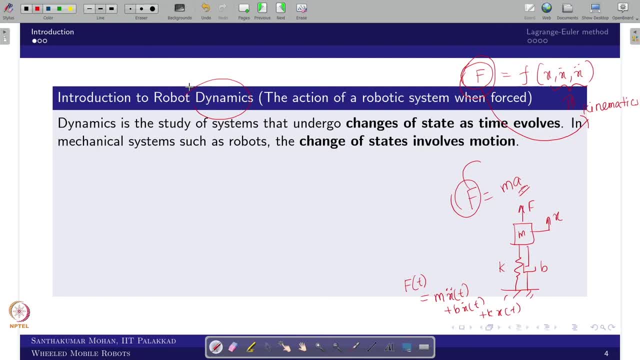 when forced The force in the sense, do not see only force, So forced means it is a general, you are giving some input, So in the sense what you are trying to see. So the system will definitely will change of state as time evolves. So in mechanical system Such as, 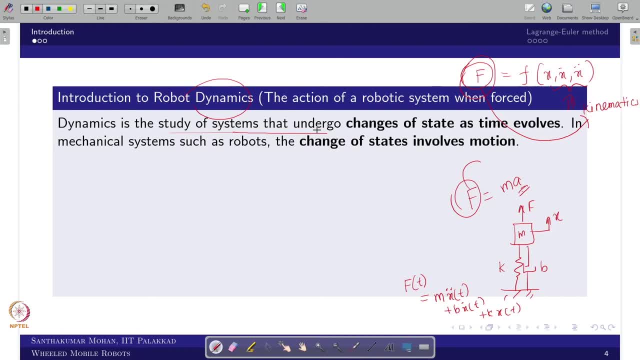 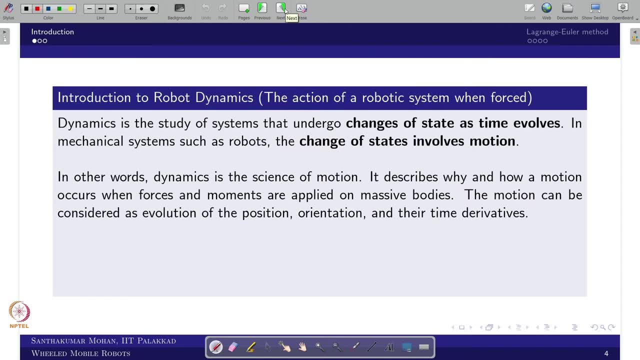 robust. what you are say that change of states involves motion. So with respect to the change of, you can say, inputs, that is what we are trying to see. So in that sense, what you can see, this is also one kind of science. But what we are really interested to see this why you need to know the robot dynamics. I 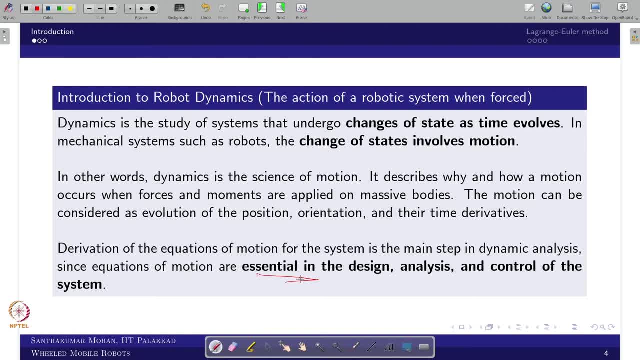 already gave a glimpse in the very beginning. So this is actually like going to help in design the overall system where you can design your mechanical, you can choose or select your actuator, or you can actually like design even the control system and along with navigational aspect. 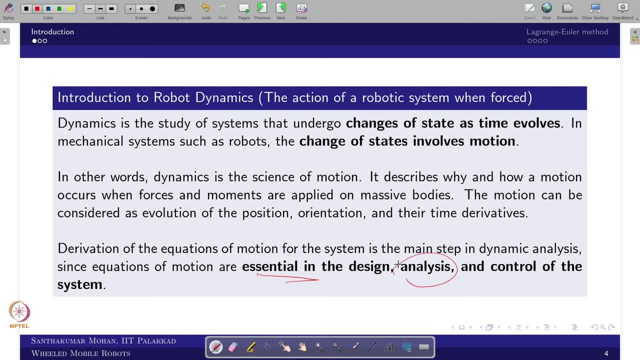 Further what you can see, you can analyze. that is what the aspect, So in the sense the dynamics is actually like one of the important case. So here the dynamics would be broad into two. One is motion dynamics, other one we call structural dynamics. 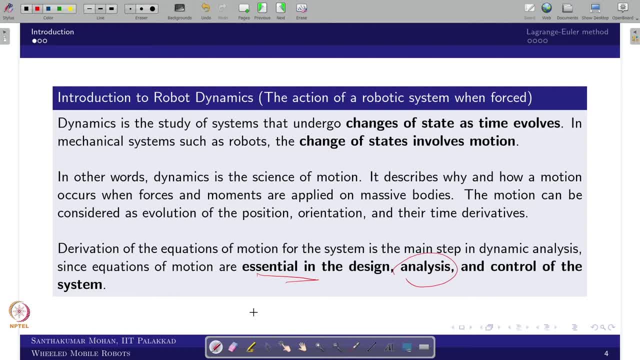 This particular classification. not everyone will do, But most of the robotization will do, Because the motion dynamics What we are focusing in more in the. you can say robotics course, What that mean, equations of motion. So when you talk about the motion, 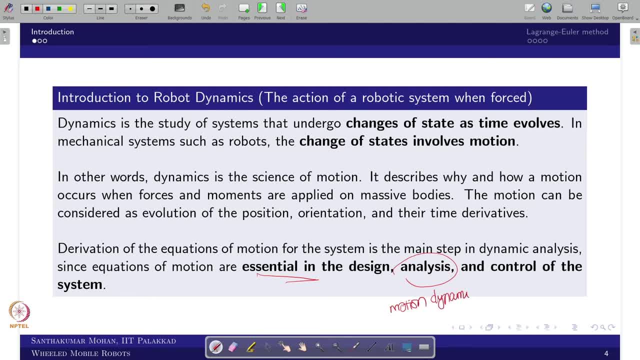 So the motion dynamics is actually like one side, So the you can say contemporary would be the you can say structural dynamics. So the structural dynamics is actually like where you take non moving entities But the moving entity. it is actually like going to give a set of equation. 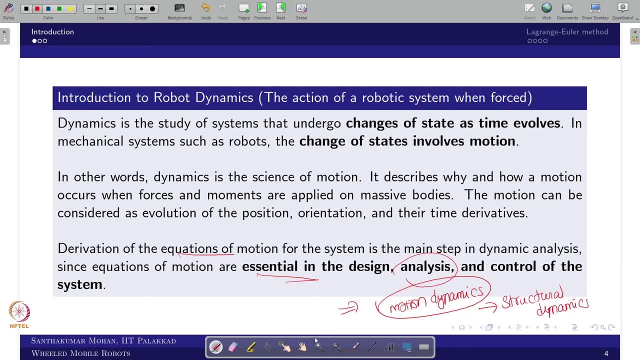 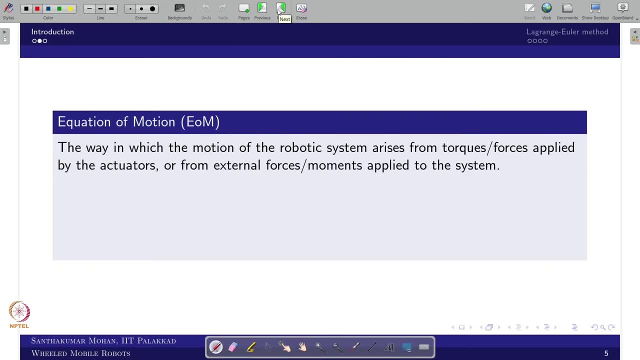 That set of equations, What we call Equations of motion. That is what we are trying to derive in this particular lecture 11. ok, So now you are clear what we are trying to see in this particular lecture. Let us move further what I said already: the equation of motion. 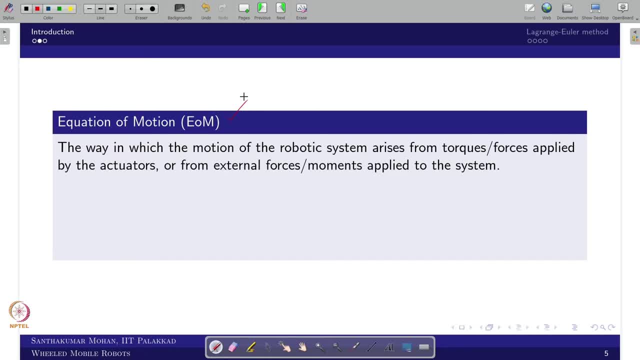 If there are several equations we call equations of motion. So this is what we are trying to write, as I already given a glimpse. So this is what the overall form where f equal to you can write: mx, double dot plus bx, dot plus kx. 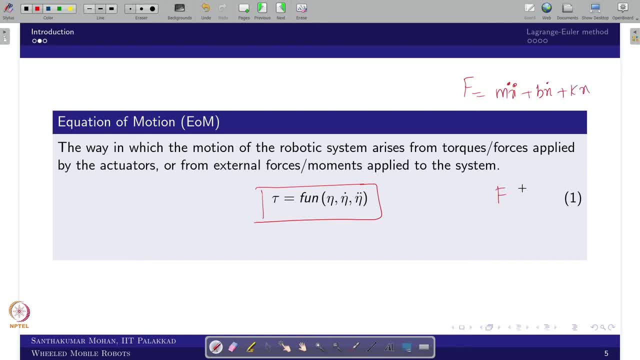 Where you have written this I can rewrite as f in the function of x, x dot and x double dot. This is a scalar. Now we are bringing it as a vector. Then that vector I am calling as a tau. this is a vector where eta is what you call system. 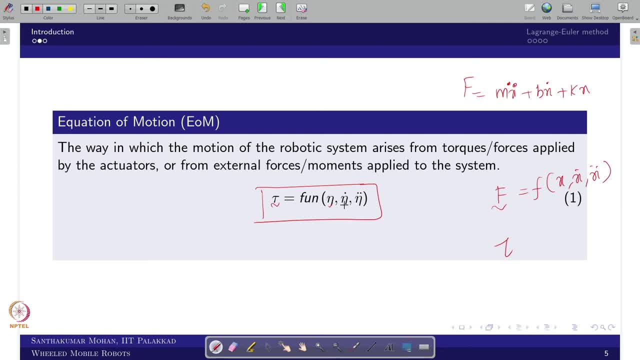 state generalized coordinate that would be having and their derivatives are given. So now you can see like some aspects have come already. So one side, there is one input, So the other side is actually like the response for the input. In the sense This is action and this is the reaction. 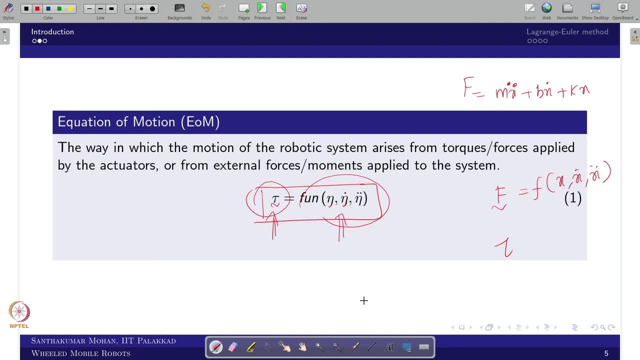 So we are trying to see the relation between action. what would be the reaction at the system level? So this is what you call equation of motion. So why this is so important? So you can do two subset of the dynamics. that is what we are trying to focus. 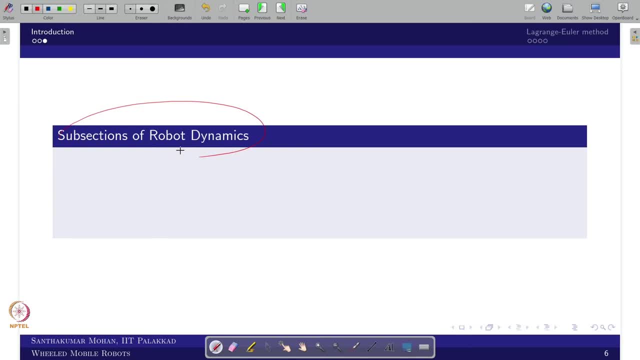 So what that? so you can see like the subsection of robot dynamics, as what we have seen in the robot kinematics. So what, the robot kinematics aspect. So We are trying to see that, if you know the input and you are trying to see what are the 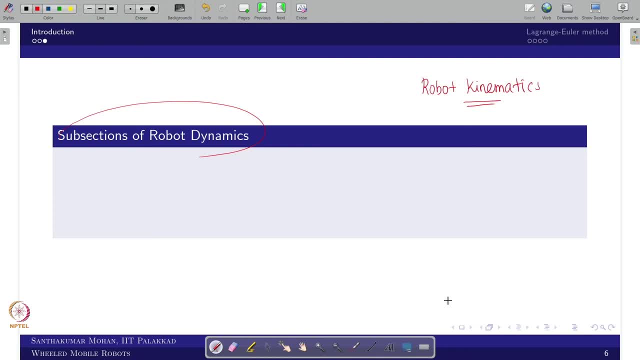 study of you can say the motion, That is what you have said as a forward differential kinematics, Whereas you need some decide system, state how you can actually like you certain input so that you can achieve that. that is what you call inverse differential kinematics. 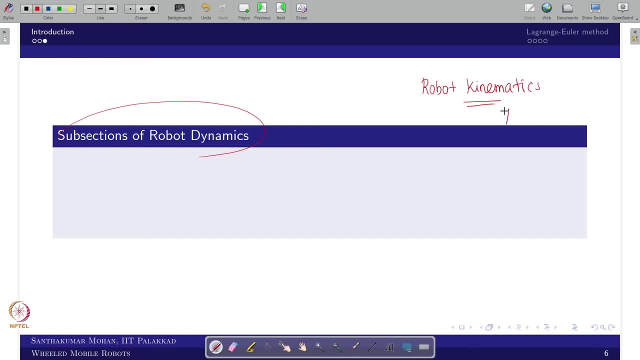 There you have written. you just recall the equation. So you have actually like written eta dot as J of psi into zeta, right. So this is what you have actually like up time, but what you can actually like. see that if I know this input command, I can find the. 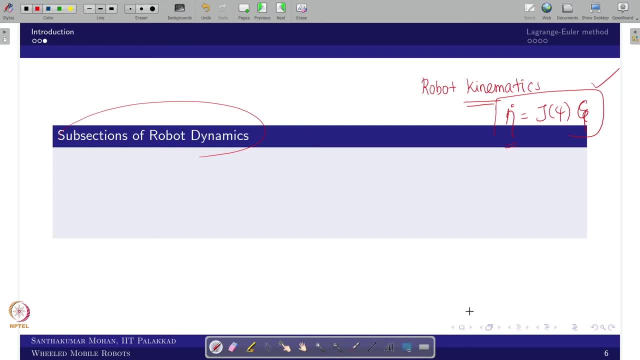 eta dot or the other way around: eta dot, decide is given, I can find what would be the necessary input, The similar direction, what would be the two subsection. so one would be forward, ok, so the other one is inverse. So then, by looking the equation itself, you can see. so this what you have written, so 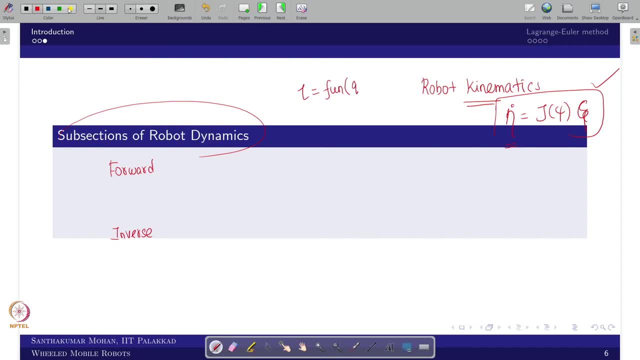 I will write: ok, eta, right, so that is what we have actually like taken at. so this is eta, eta dot and eta, double dot, right. So. but now, looking at here, this side, right hand side, we have given as a input. based on that, you have taken a forward and inverse, but here it is not like that. 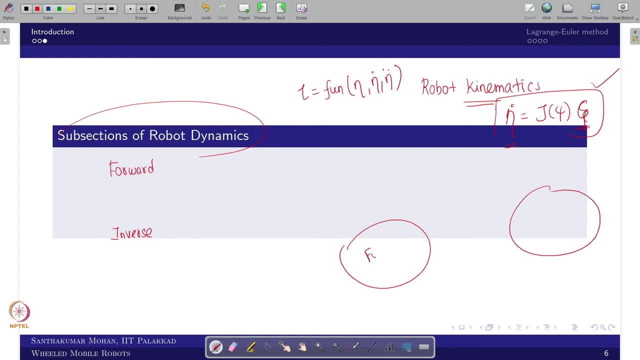 So what? you have two spaces, so one is actually like your force and moment. so which is I call? So this is the general as a cause of motion. so these are the causes. So the other side is actually like motion, variable, in the sense you call eta, eta, dot. 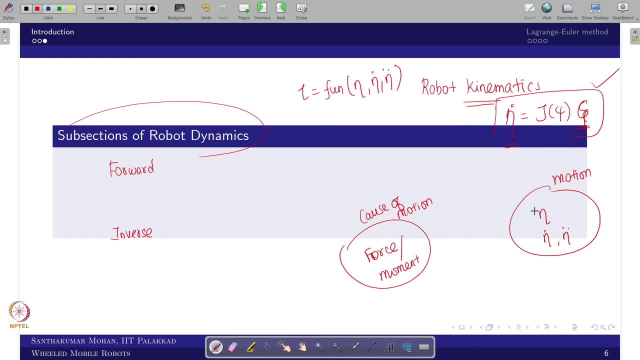 and eta double dot in the sense position, in the sense displacement, velocity and accelerations. So now we are trying to map these two- if I do the mapping ok- from the known forces and moments. in the sense I connect the wheel, I give a desired task, in the sense I take. 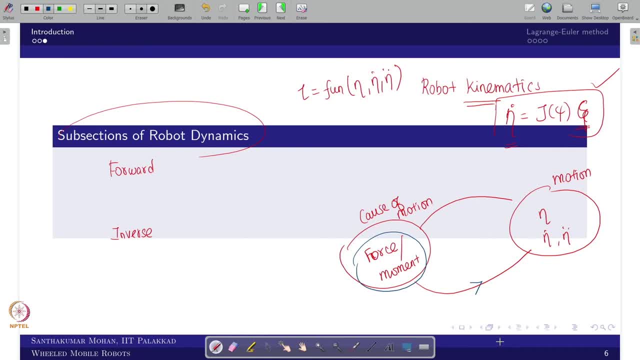 a proper rotation So that I do, then that is what you call forward dynamics, whereas I am actually looking the other way round. I am giving everything as desired, in the sense earlier what we have seen, position trajectory, but now you are giving actually like what you call the general. 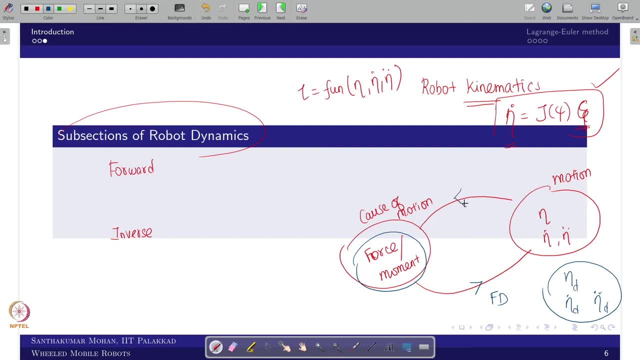 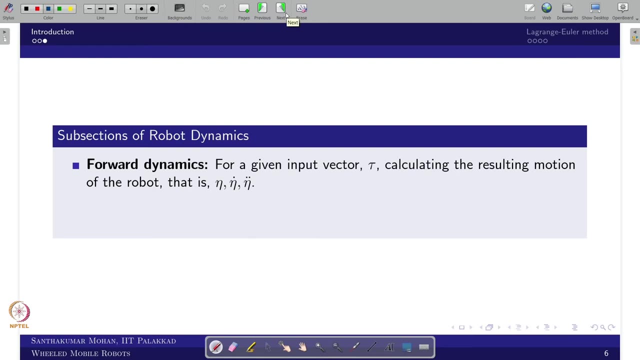 trajectory, if I actually like, do this given and I can find the forces and moment. so that is what you call inverse dynamics. So you can actually like, by looking itself. This is nothing like analyzing and this is, like you can say, controlling. So that is what I put it in this particular slide. you can see forward. dynamics means: 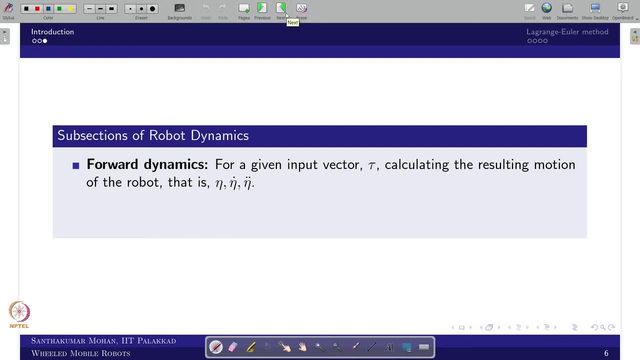 for a given input vector, tau, calculating the resulting motion of the robot, that is nothing but eta, eta dot and eta double dot, whereas the inverse dynamics is nothing but So. for a given desired trajectory, where eta, eta dot, eta, double dot, all desired and try. 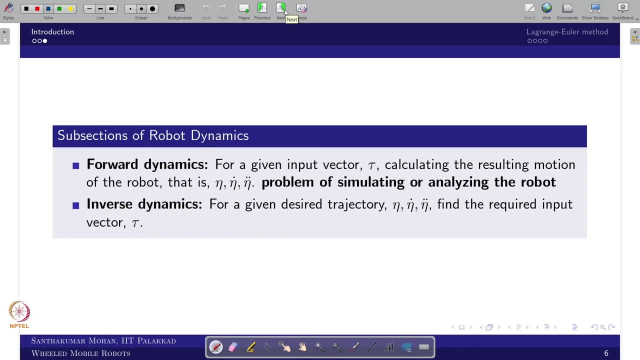 to find out what would be the input vector tau. So So that is what we are actually like looking at. So one what we call problem of simulating what we did in the you can say kinematics: the same way it is simulating but in a you can say dynamic level. 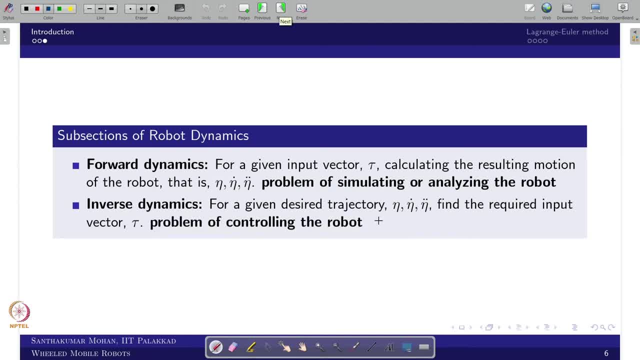 So the other one is actually like controlling the robot in dynamic level. Again, I am giving a disclaimer. So control means: do not see, it is a feedback, it is a open loop. ok, So very specific, it is a feed forward. So I do not want to give a state forward terms now, because we are trying to cover these all. 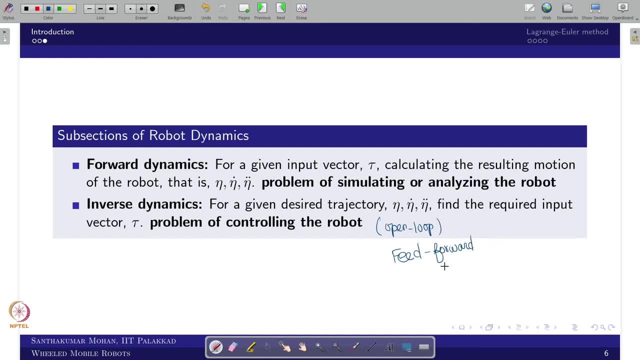 in the What you call the motion control, but this is a feed forward control. ok, So similarly what we did in the inverse differential kinematics: the same thing: feed forward, where you are not taking any feedback, you are just giving whatever you calculated that you are. 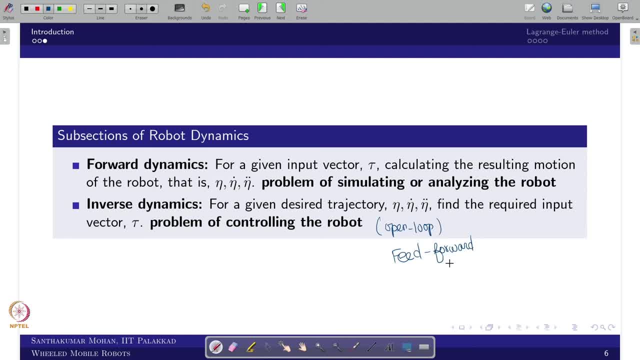 giving as a input. So now we will actually like see how to derive this. So there are several way. ok, there are several methods. So there are two popular methods in robotics which we commonly use. one is actually, like, based on energy. ok, 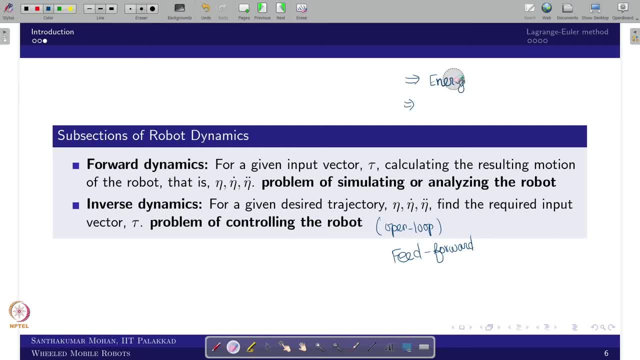 So I will just Ok, So I will just make it. So one is actually like energy, So energy based. So the other one is actually like a simple what you call force moment base, So I can actually like say that that is a momentum. 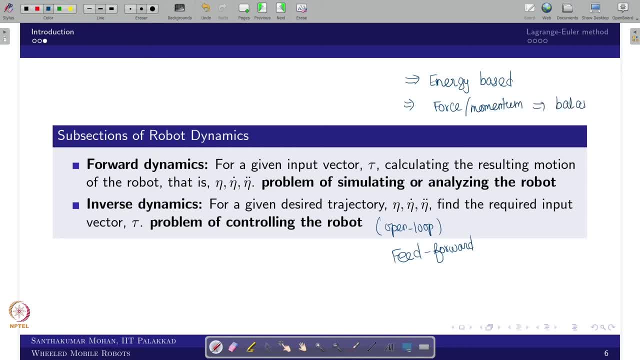 So force momentum base, in the sense it is a balance approach, or you call equilibrium base, Ok, Ok, Ok. So the other one is energy base. In this particular lecture 11, part 1, we are trying to see the energy base. So you know, energy equation. 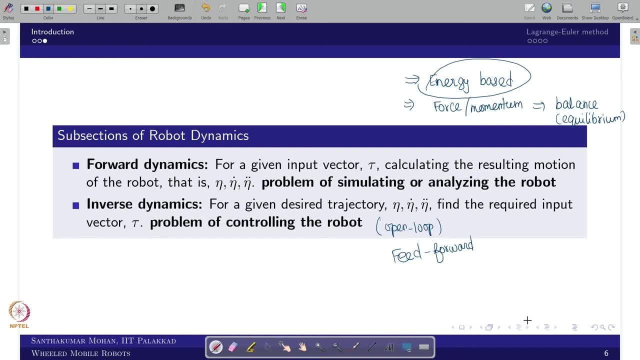 So we are actually like modified the energy equation by Lagrangian, or you can say Lagrangian, So that equation modified equation, what you call Lagrangian, and this energy equation given by Euler modified one equation. So the Lagrangian has modified the Euler equation into further. 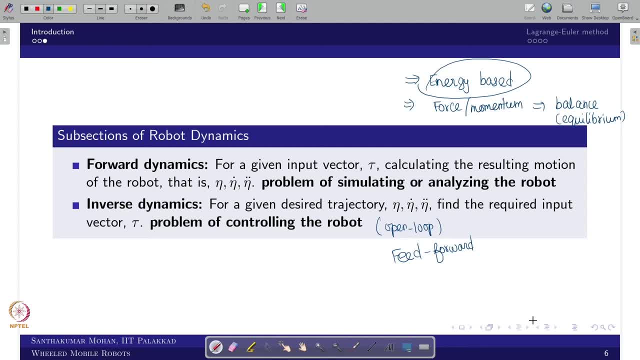 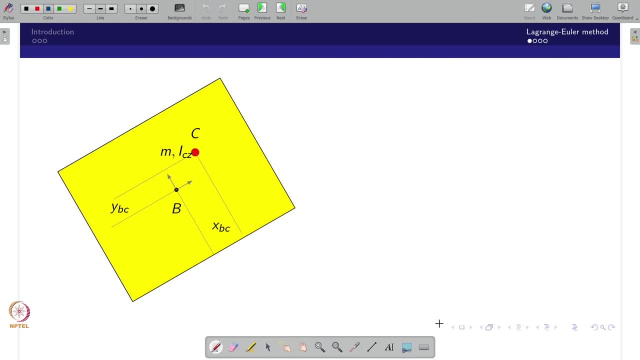 So that is why it is called Euler Lagrangian equation or Lagrangian Euler method. Ok, So that is what we are actually trying to use. for that, again, I am bringing back to the original. So the mobile robot I am assuming as a rectangular box, where this is the body frame, because we 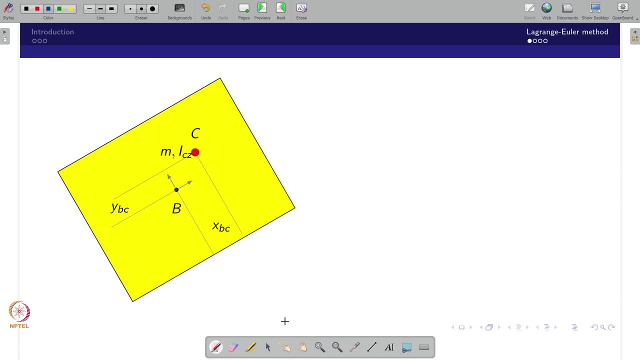 cannot always assume that the body frame and the wheels and you can say the vehicle centroid would be aligned. So now I am taking a very general case where the body frame is here but the centroid of the vehicle in such a way that you assume that the mobile robot is, consists of several. 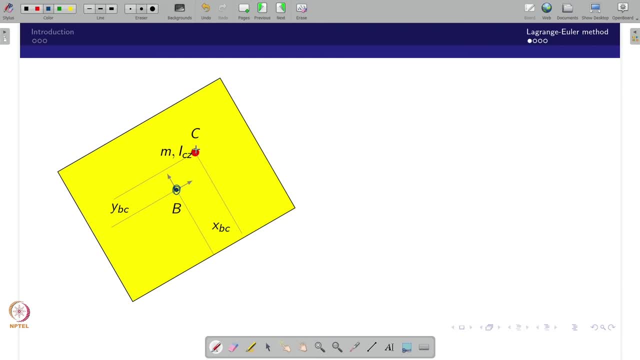 batteries and the payload. The CG is actually like move away from the body frame. So then what would be the scenario? So now you see that now we brought the mass, in the sense you brought the inertia, So the linear and the rotational inertia you brought it. 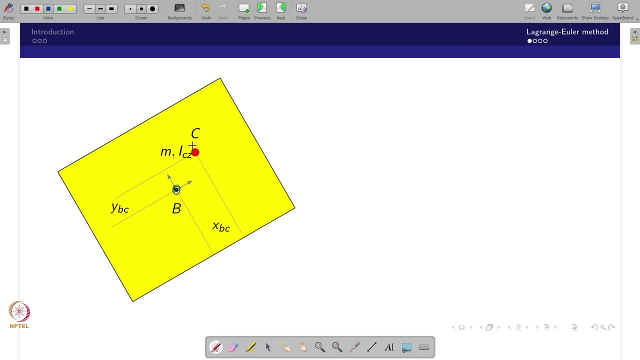 So then what happened the centroid point will have as a lumped mass and lumped inertia, we can realize. So I am just giving as a disclaimer. So the I is, you can say, a tensor, but here I am taking, since it is moving in a XY plane. 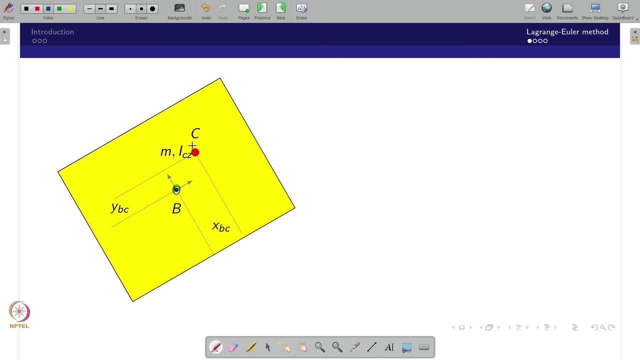 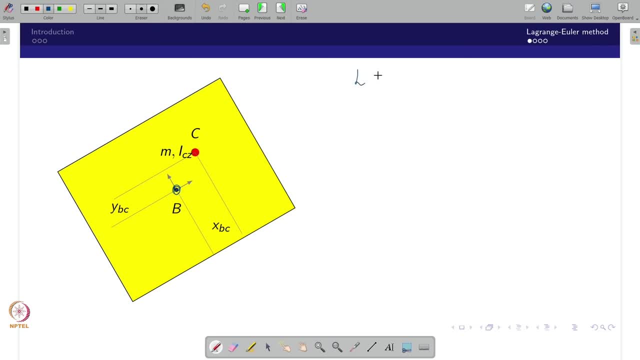 So the Lagrangi said that if there is a energy difference, then there is a motion exist. Then the motion exist means can we use a energy method? yes, So what? the energy method says that. so the dou E by dou, I call V whole. this is a actual 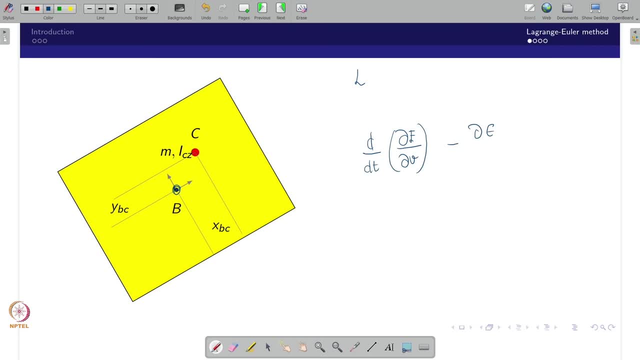 like going to give a momentum equation. So this would be dou E by dou L, So this would be dou X would give 0.. Ok, This is what the energy equation, But what Lagrangi modified is. So this would happen when there is a energy difference. 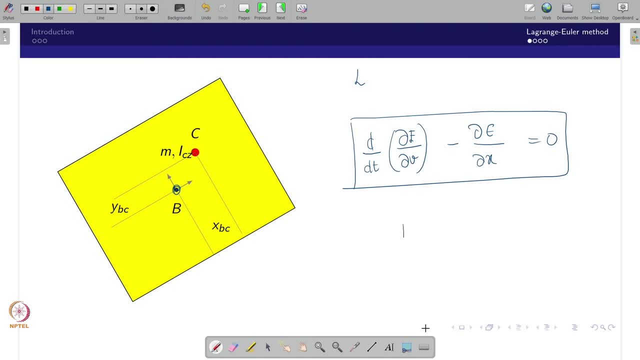 So the energy difference here? it is a rigid body, we assume. So in the sense, what are the energies? would be there? only kinetic and potentiary energy. in the sense you take kinetic energy minus potentiary energy, this energy difference exist. then there is a motion exist. 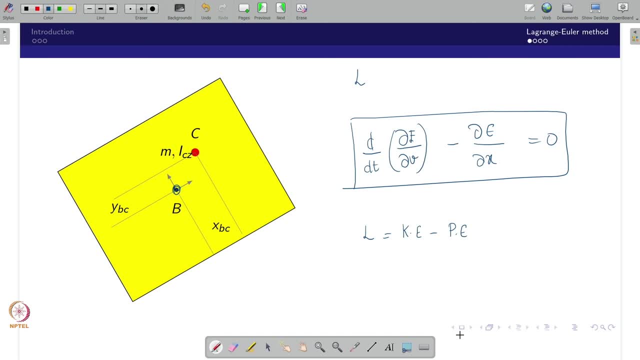 So, for example, you take a simple pendulum. So when the simple pendulum start oscillate, you assume that it is a rigid body. there is no spring attached. It is a simple rod attached with the, you can say- hinged point. So now, when the pendulum will start oscillate, you take the point away from the equilibrium. 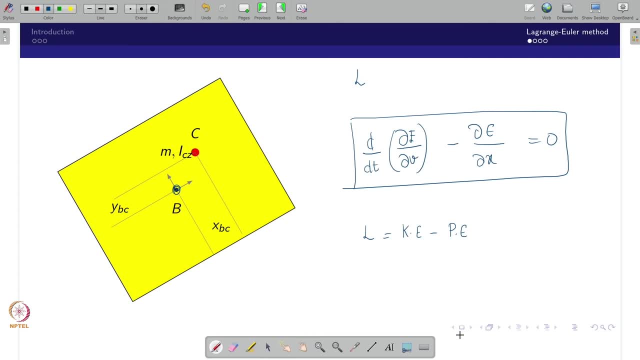 So, then, what you are trying to induce, you are giving a potentiary energy, or what you can see, that the bar which is hanging, you just hit it. What you are trying to give, you are trying to give a kinetic energy, either one or combination of this. 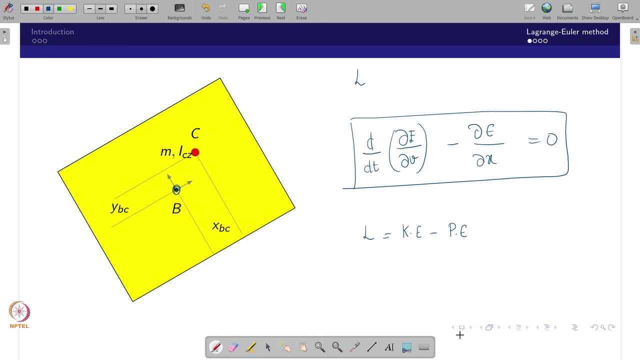 So there is a energy difference, then there is a motion exist. This is what Lagrangi gave. So now what? Lagrangi modified this Euler equation? So he modified this d by dt. So doh l he brought and doh v still exist. 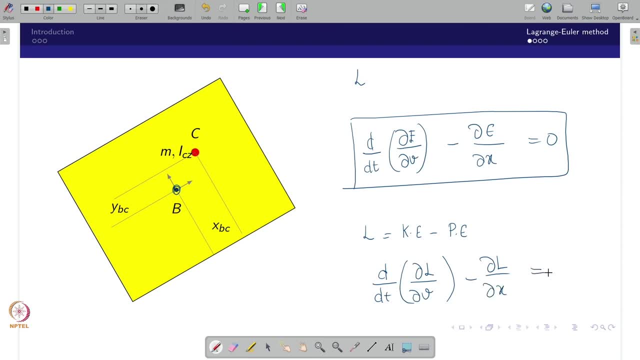 So doh l by doh x, this is equivalent to the applied force or torque. So this is what we have actually like, seen. So this particular equation we are trying to use. So, in the sense, what you need, You need kinetic energy of the system. 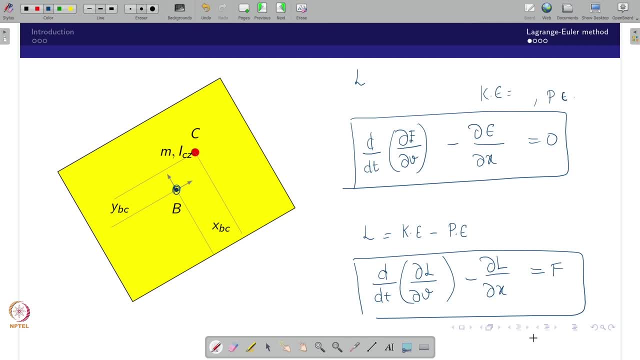 Okay, Then you need potentiary energy of the system. Fortunately the mobile robot or land based system. we assume that the potentiary energy is constant, and that is. we even assume zero. Why it is so? Because it is moving on the land, so the gravity effect would not be there. 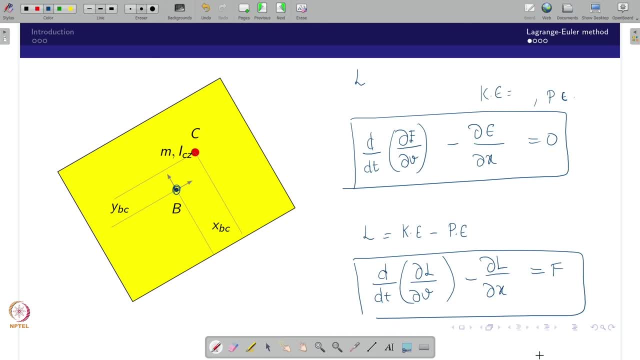 Okay, If we bring the suspension- that too, like we assume that multi body approach we need to bring- but right now we assume it is a rigid body, that too like a lumped mass system- Then this all will go as it is. So in the sense, 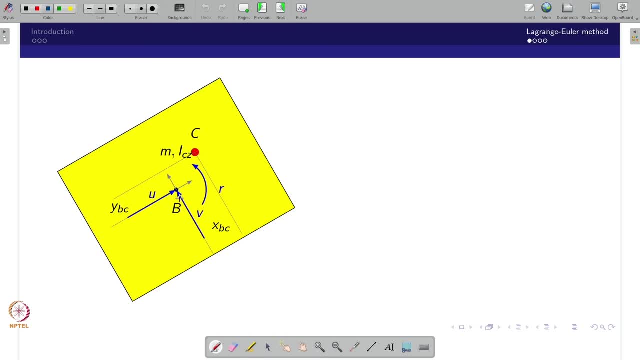 So you can see, the body frame would have a linear velocities u v r. this is what we have seen in the kinematic aspect. In addition to that, what we have brought it, the displacement or you can say the distance between b to c is x b c in x axis, y b c in the y axis. 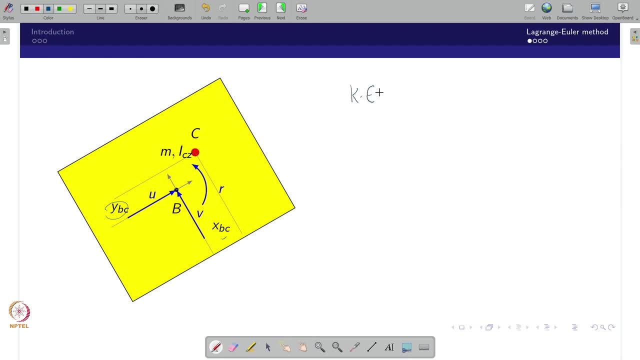 So now, what we are trying to see, We are trying to find out the kinetic energy. What would be the kinetic energy of? Okay, So the mass. So there are two kinetic energy would be there. There is translational kinetic energy, which is due to the mass. 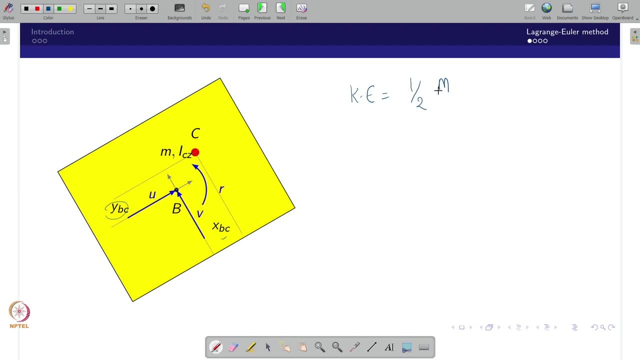 There is a, you can say, rotational kinetic energy due to the rotational inertia which is we call second moment of inertia. So in the sense it is supposed to be x c dot square plus y c dot square, where x c and y c we need to define and x c dot and y c dot need to be defined. 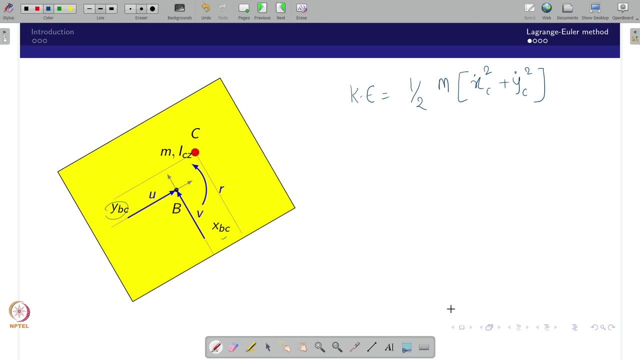 We have already taken. this is actually like instantaneous velocity: u, v, r. So now we can actually like find what would be x, c, dot. Okay, What would be. You can see like the u would be there in the x axis. In addition to that, you can see that this y, b, c multiply with r would be opposite direction. 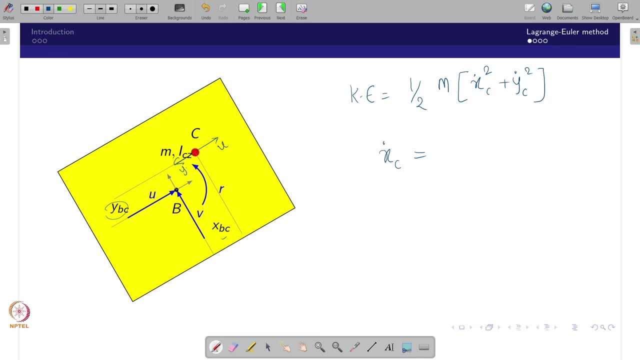 Right. So this u and the other side is actually like y, b, c, r, So in the sense, what you will have, this is So similarly, y c, dot, what would be there? So you can actually like see that this is v and, in addition to that, what you can actually 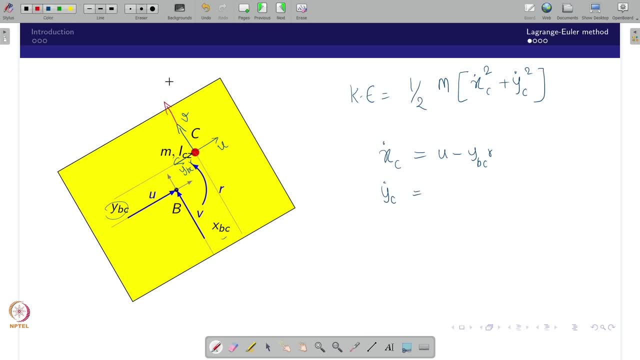 like see. So there would be additional velocity which is due to x b c. Okay, Okay, So v plus x b c into r. So, in the sense, what you can see, v plus x b c r. Alright, So now these two velocities are there. 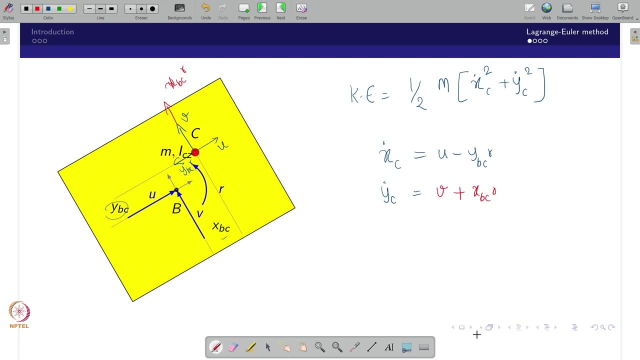 Further I said potential energy. we no need to bother because it is in the land. So now we will actually like substitute that. So this is the equation we obtained. So now you actually like put the kinetic energy for the translation mass and what would be? 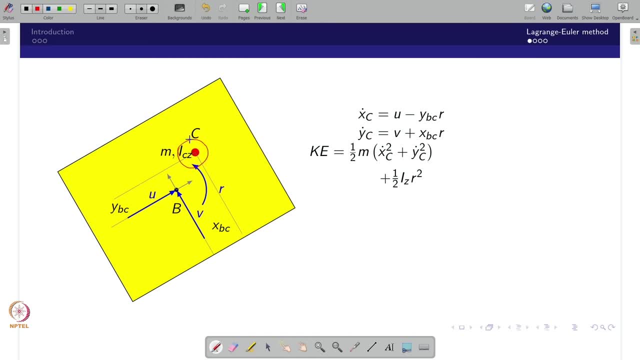 the rotational kinetic energy. There is a one inertia, which is possessed, And there is a rotational space Speed. So i c z r squared would be the equivalent you can say kinetic energy, along with half Right. So it is actually like half i omega squared in general. 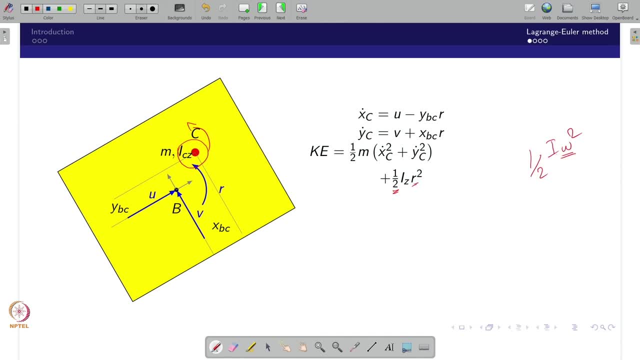 So, since the omega here is r and i is actually like a vector, but here sorry tensor, But here we assume that is only one dimensional, we are bothering. So in the sense, i z comes and the remaining is coming Right. So now what you got it? 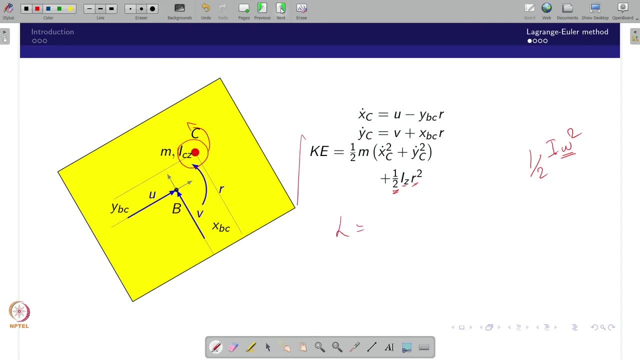 The kinetic energy. you got it. So what would you substitute in a Lagrangian equation? What would be the Lagrangian equation? So kinetic energy minus potential energy. So this is the equation. So in the sense, the kinetic energy is the nothing but your Lagrangian. 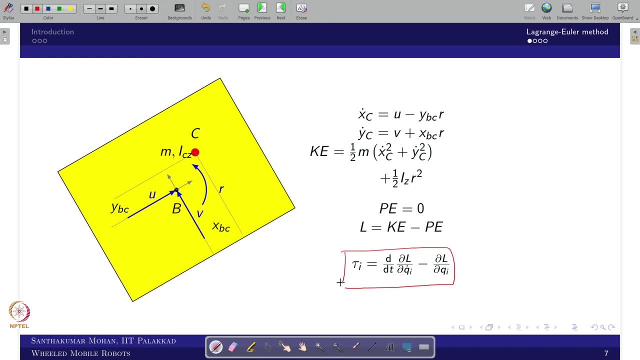 And you take the Lagrangian Euler equation and you do it. So what are the equation you wanted? So what would be equivalent in the x axis force? What would be in y axis force? What would be in the z axis moment? Right, 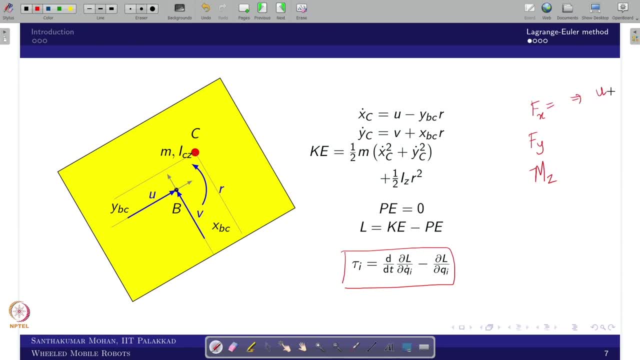 So now this would be actually like related to the u and ud Right, And this is related to v and v dot, and this is related to r and r dot. So what dot? It is nothing but acceleration Right With respect to body frame. 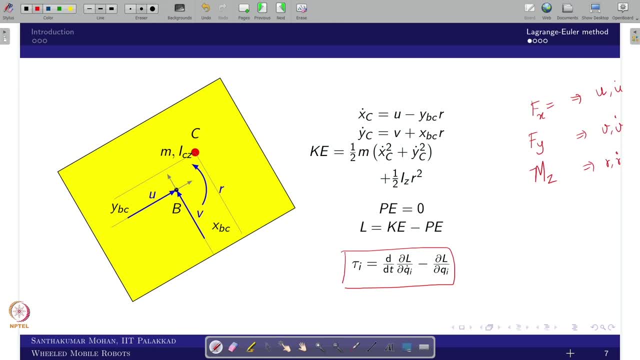 So this is what we are trying to derive it here. So for that, the first one is: we will actually like take it this, So we will actually like move forward. So what that means actually like we will actually like take this and we will actually like partially. 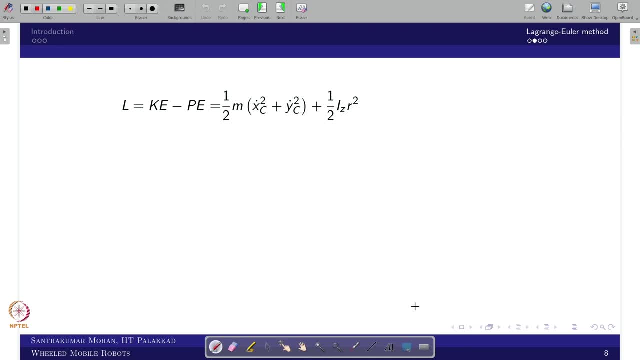 take the differentiation with respect to you. call u, Then we will take v and take r And we will actually like try to take the time derivative. that is what I am doing, it one by one. First, I write the bigger equation in the sense I expand this xc dot and yc dot in the form 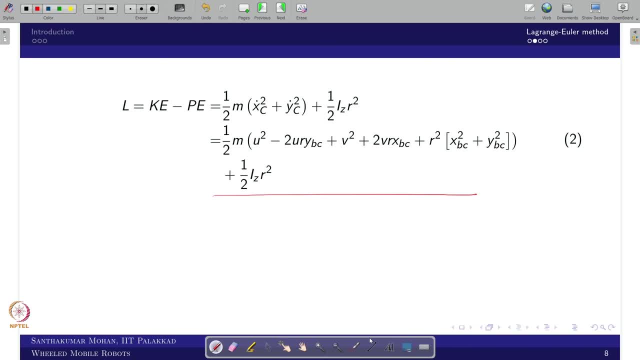 of u v r, and I am actually trying to substitute and actually like square it, and I am making you this equation. Now, what we are trying to do, We are trying to take the dou L by dou u, So dou L by dou v and dou L by dou r. 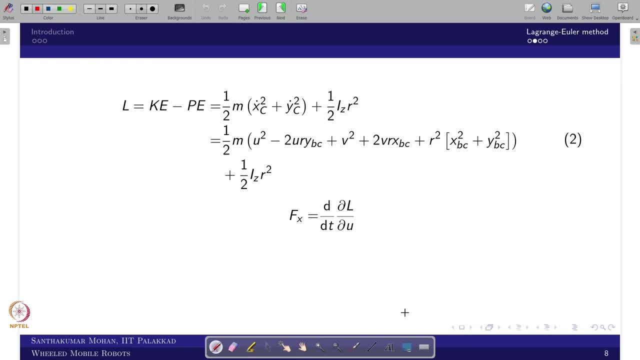 Right. So this is what I am trying to do. So first I am trying to take fx. So since dou L by dou integration of u is not there, Why it is not there? Because we are seeing everything in the body frame When we are seeing with the inertial frame. that is what we are trying to cover in lecture. 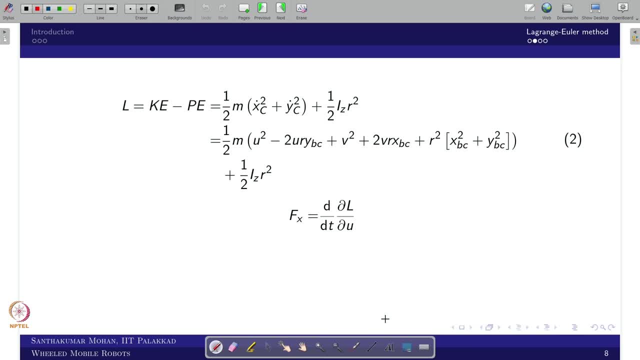 12. So then everything will come. Right now we are taking everything with respect to body frame. Why it is so? Because the wheels are attached with the body Right. So that is why we are trying to take directly as fx with respect to body. 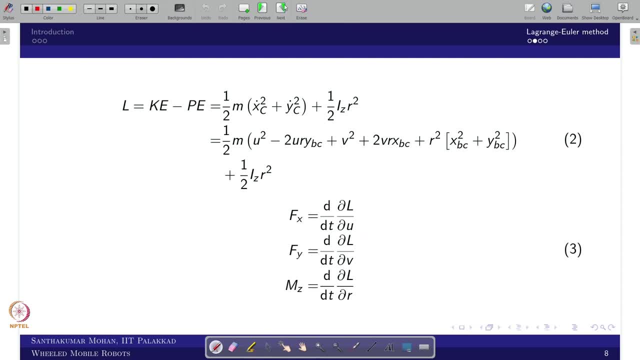 So now this is what the equation, Similarly So fx and mz. you can get it Already. you know like what is L. You take the partial derivative with respect to u. So that is what we are trying to do in the next coming slides. 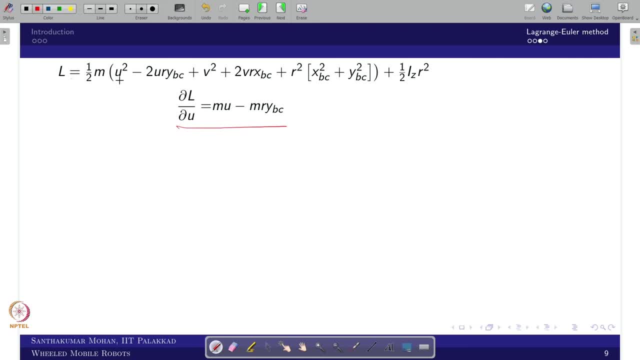 So you can see like this is what happening: You take dou L by dou u, So this term will there. This term is there, So remaining all the terms are 0. Right. So similarly, you take dou L by dou v. You can see these two terms are not having any v term, only these two are there. 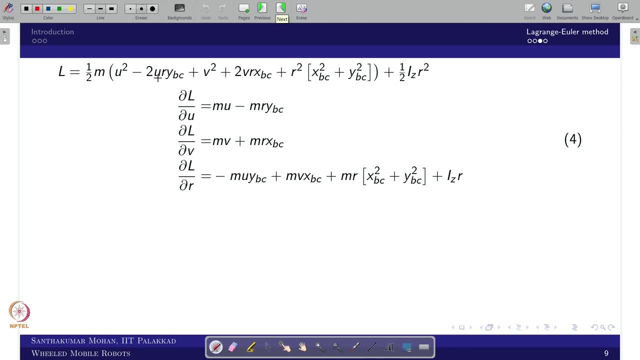 So then you can take dou L by dou r, Right, So you can see: r is here here and here Right And here also Right. So now, what you got it? You got it dou L by dou u, dou L by dou v, dou L by dou r. 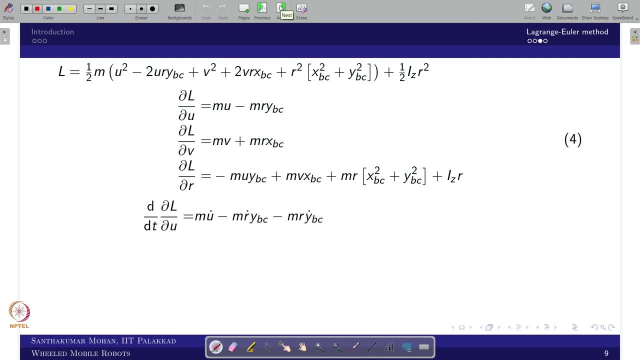 So now you take the time derivative that is equivalent to fx, fy and you can say mz. So that is what we have done Right. So you have taken time derivative of this. So u also function of time, r also function of time and ybc also like function of time. 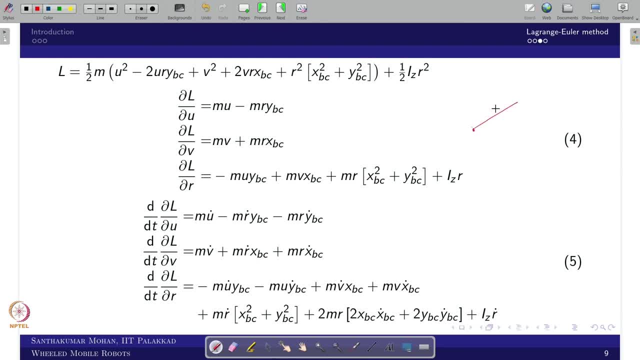 Why it is so? Because that is actually like moving with respect to, You can say, body, So the body is having a longitudinal velocity. So now this ybc dot and what you call xbc dot are equivalent to xc dot and yc dot. 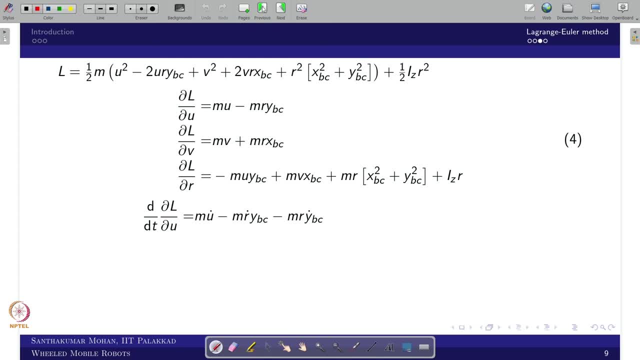 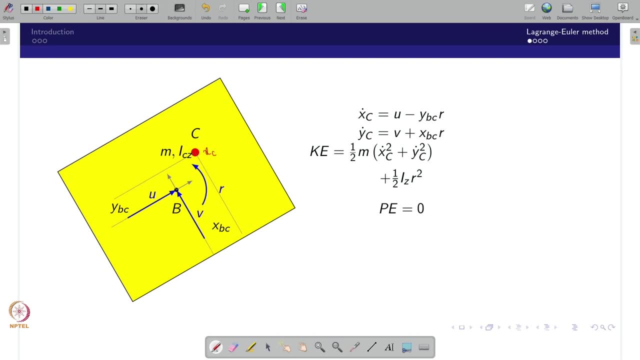 So why it is? so Because if you look at the picture then you will get idea. So I will. you can see like what this equivalent. this is what you call xc, xbc, Right, Ybc. So if you take a time derivative, what it is equivalent. 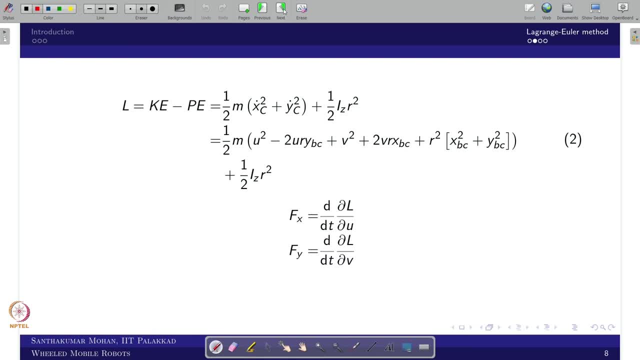 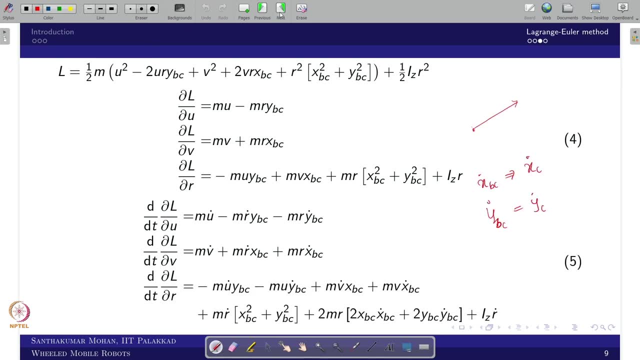 That is equivalent to this Right. So that is what we have actually like taken here. So now you can actually like see if you take a time derivative. So these all actually like going to come and you know already what is: ybc, dot, xbc, dot. 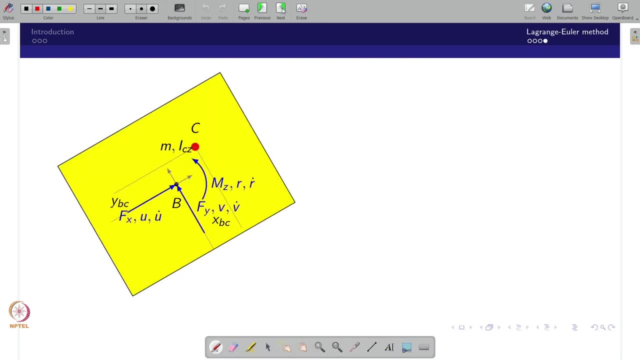 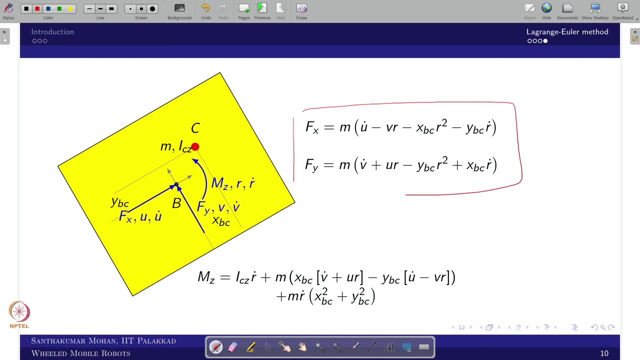 So then you substitute, you will get the final equation. So that is what you call. you can say fx, fy and mz. Okay, So now you can see that this is the equation we obtained for x axis force and y axis force, And this is the moment. 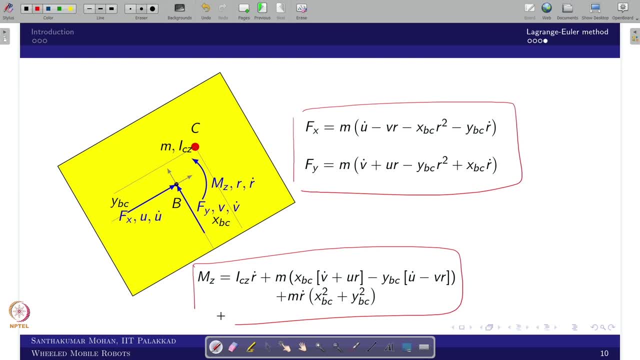 So once you obtain, you can just recall, So what you have studied, So you have studied in, you can say: simple case. I assume that. So this is actually like r and this is theta. So this point I am calling P. Okay, The P I can write as r, e power. you can say j, theta. 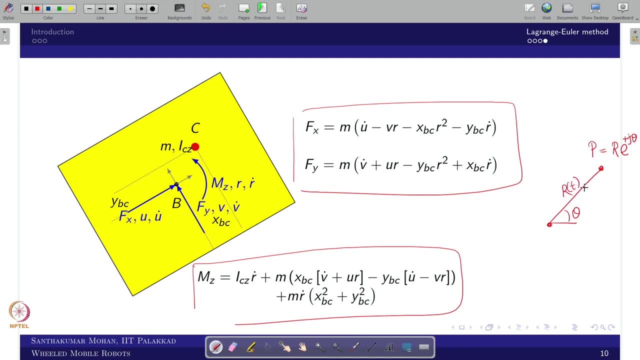 Right, So now you assume that this is also varying with respect to time. This is also varying with respect to time. Okay, So what is the P dot? So P dot is actually like r dot of t, So e j theta plus. you can say r of t, r of t. then you can say like e j theta of t and 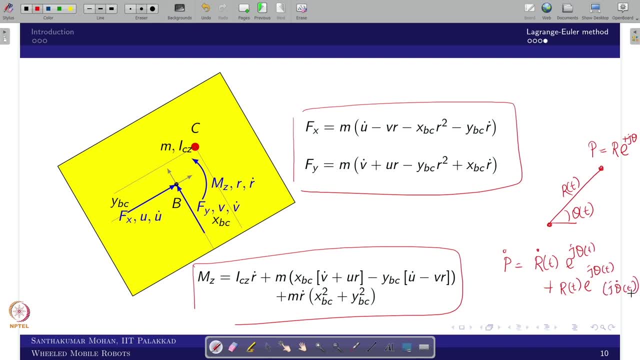 then j theta of dot Right, In the sense what you will get first you will actually get this value. then it is something like e a power, x differentiation with respect to x. So what you will write, So a e power, a x Right. 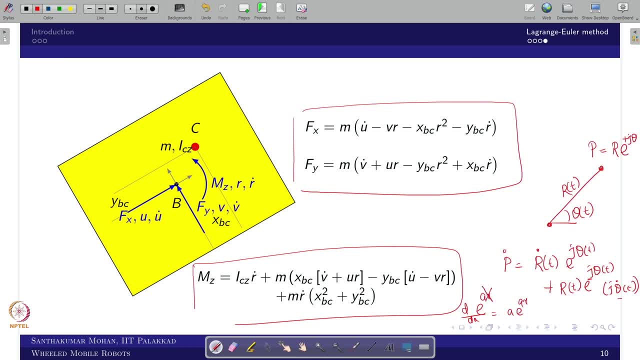 So that is what we have written, but right now it is a big x, So then you will differentiate that. So in the sense, what one can see, this is actually like j is coming Right. So now you take the P double dot term. 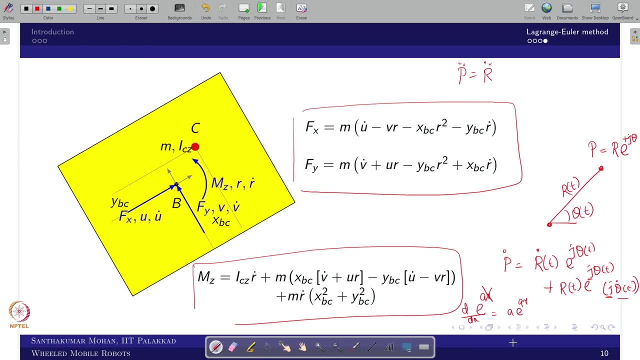 So what you will see. So r double dot also will come, Then r dot term along with you can say theta dot will come. Then you can see like r multiply with theta, double dot term will come. Okay, So this is actually like j. 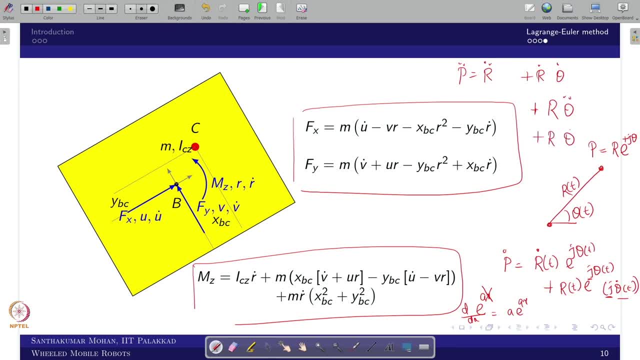 Right And r multiply with theta dot, square term will come. So this is what you call slip acceleration, This is what you call Coriolis And this is what you call tangential acceleration. This is what you call radial acceleration. Whether you are getting all the component in fx component or there or not, you can see. 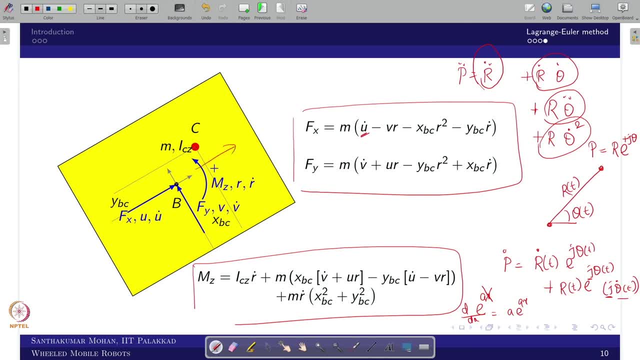 So this is, you can say, along with that direction, that is nothing but a slip acceleration. And this is, you can see, the tangential velocity, in the sense longitudinal velocity multiplied with angular velocity. This is nothing but a Coriolis component. And here you can see r squared. 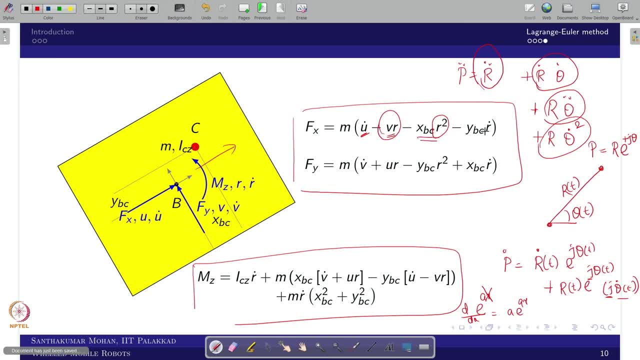 So what that? So this is a radial component. So here r dot, multiply with the position What that is Equivalent to you call the tangential acceleration. So now these are the component you can actually cross check when it comes to the moment. 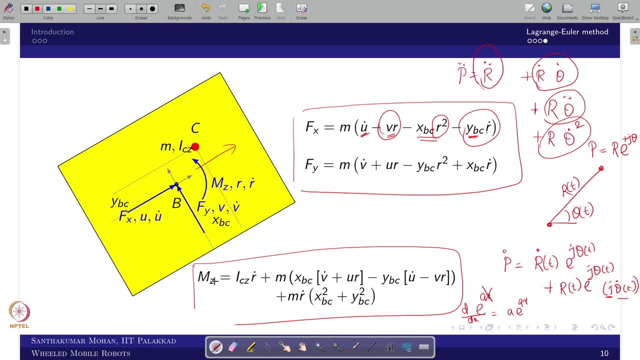 So what you call the Coriolis and other things we will actually like rewrite in a gyroscopic effect That we will discuss in later, Right. So right now you can see, like these three equation we obtained. Now we can see that the same equation can be obtained, the other method. 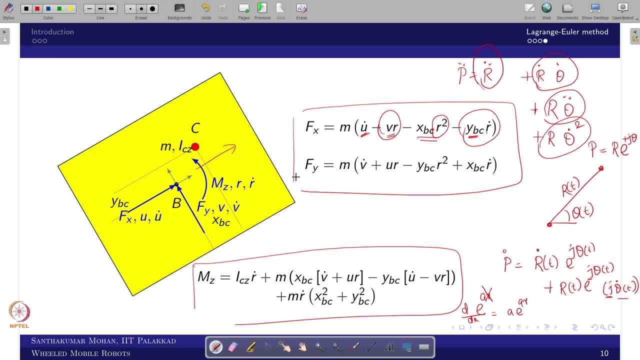 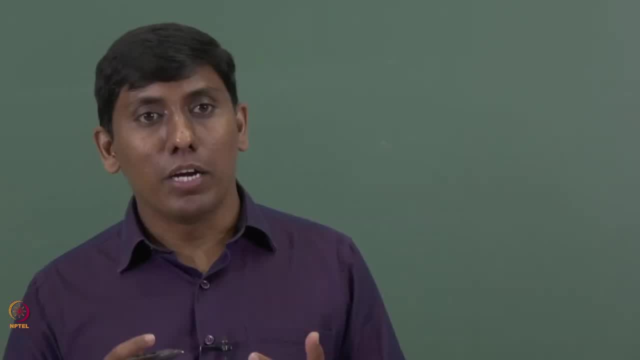 Because I told there are two popular method right. One method gave this equation, whether the other method also like, will give the same thing or not. So this is what we are going to cover in the lecture 11, part 2, where we are actually like: